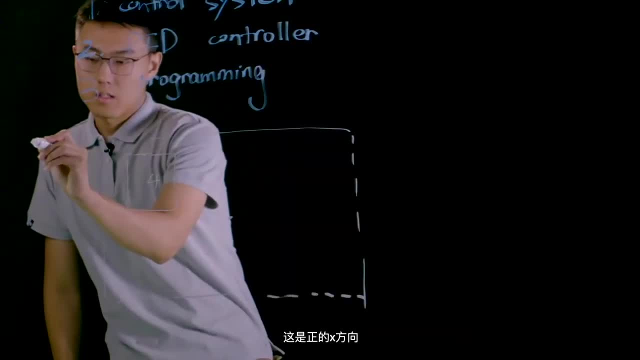 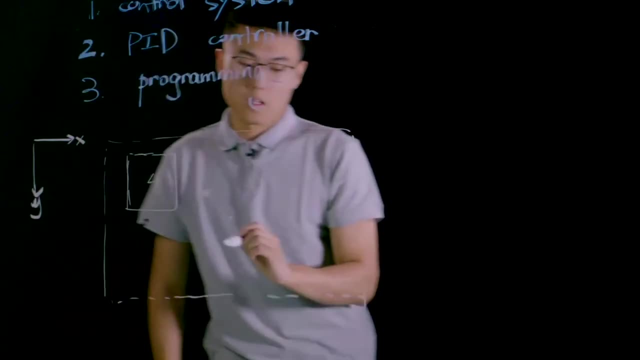 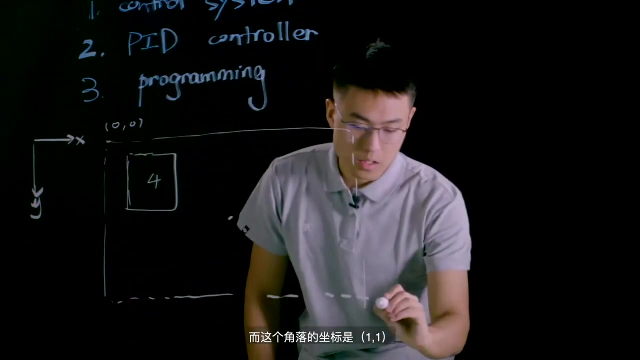 So let's say this is the position of the visual marker and the center of the viewport. Let's say this is the positive X direction And this is the positive Y direction, And this is the origin: 0, 0.. And this corner has coordinate 1, 1.. 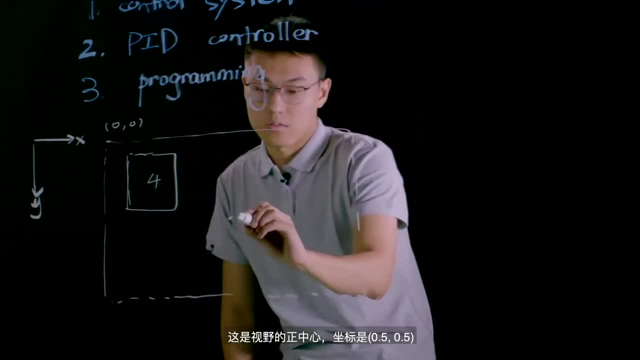 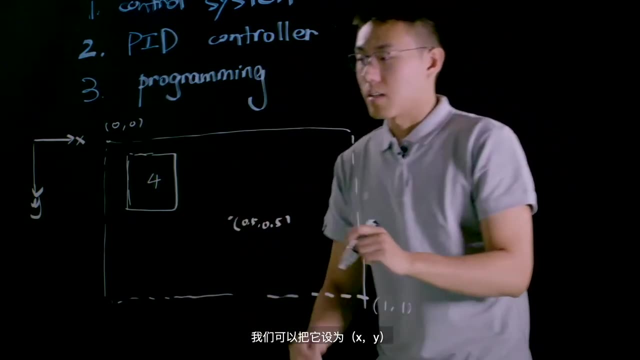 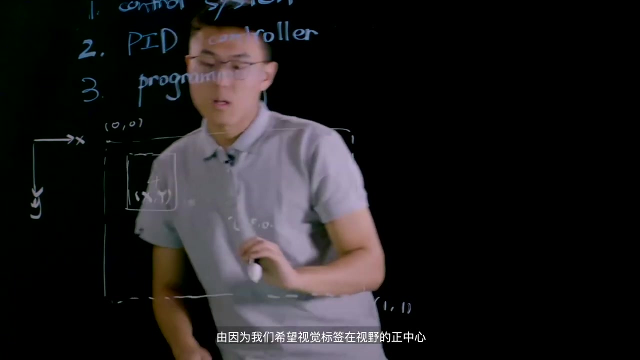 So, since this is the center of the viewport, the coordinate of it is 0.5, 0.5. And since we don't know the position of this visual marker, let's say the coordinate of this visual marker is: So, since we want to put this visual marker in the center of the viewport, 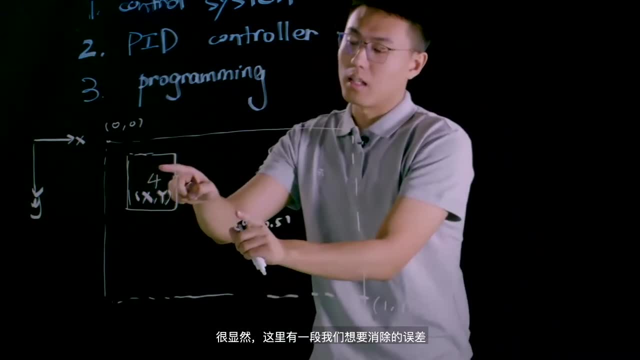 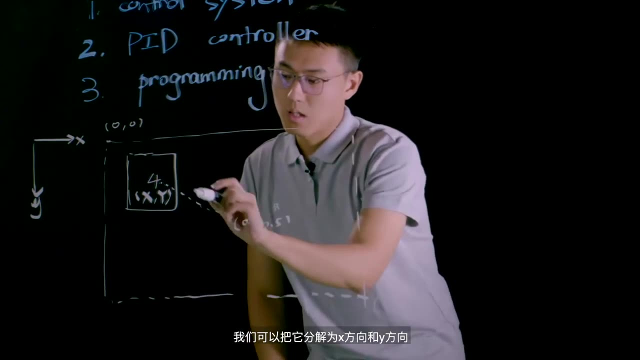 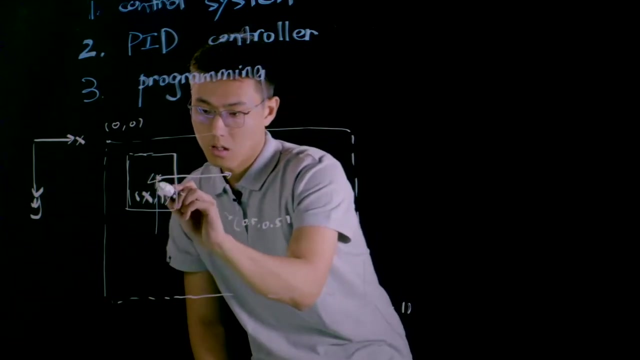 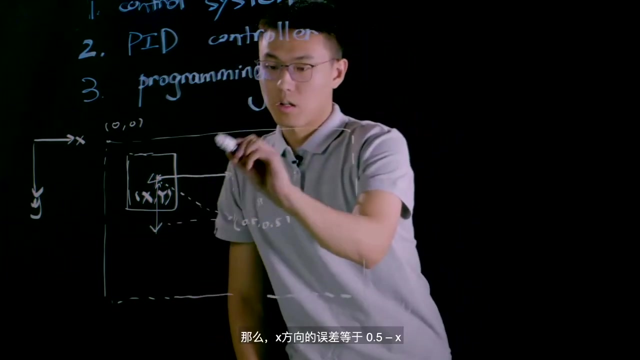 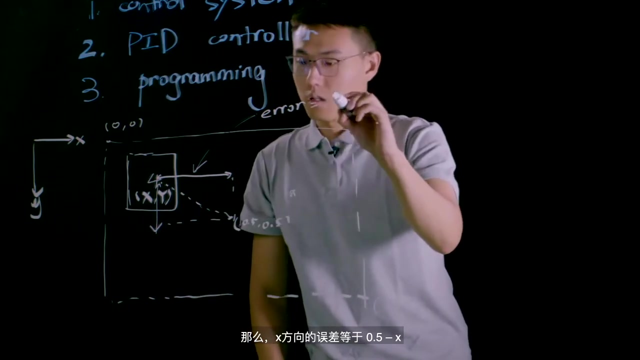 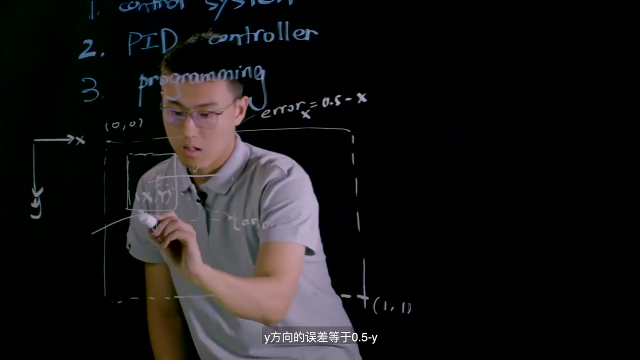 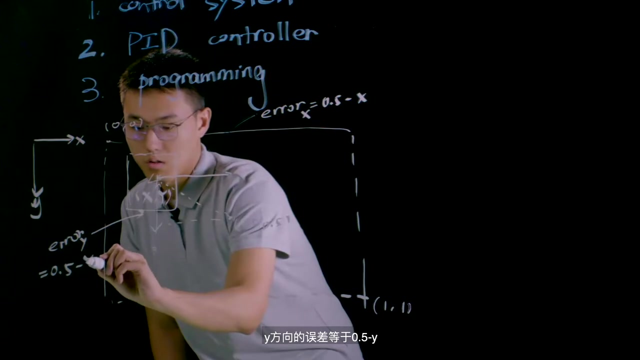 obviously this is the error we want to eliminate And we can decompose it into X direction and Y direction. Therefore, the error in X direction equals to 0.5 minus X and the error in Y direction equals to 0.5 minus y. 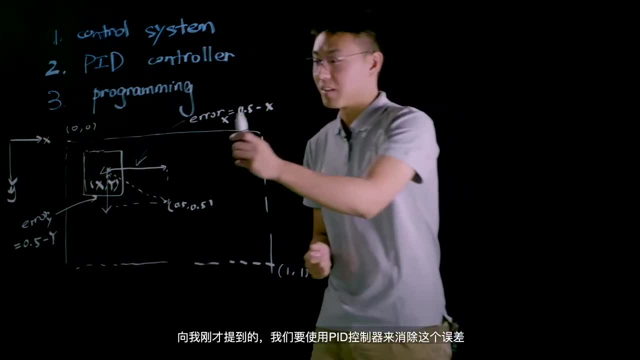 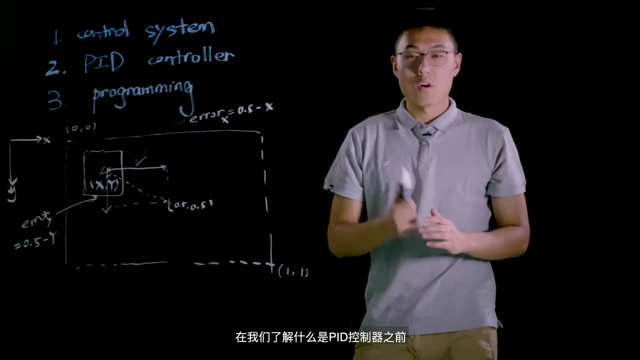 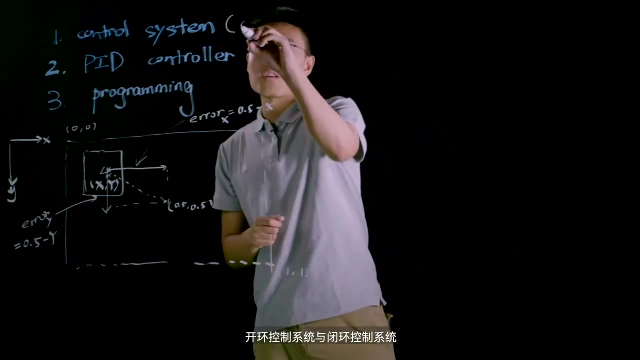 Like I mentioned before, we use PID controller to eliminate the errors over here, So PID controllers are now being widely used in modern control systems. Before we understand what the PID controller is, we need to learn some concepts of the control system, which can be either closed loop. 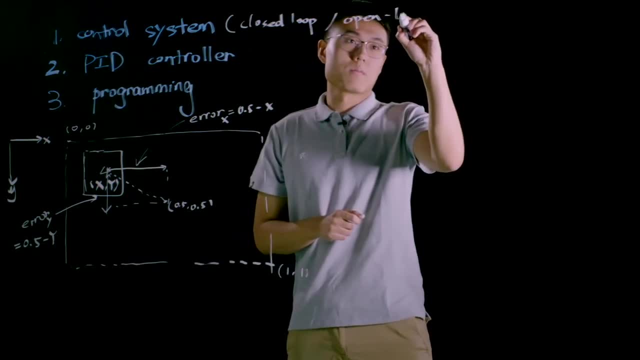 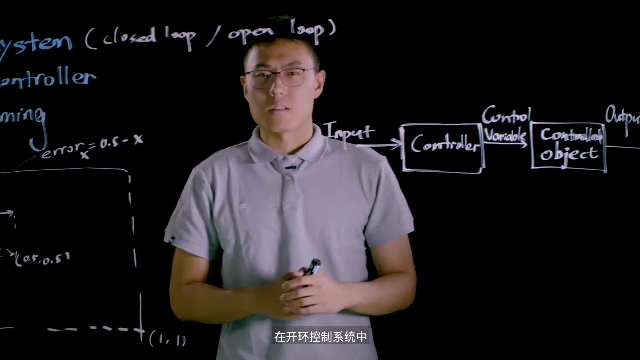 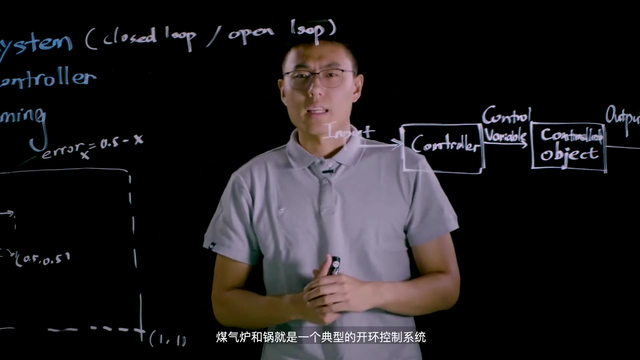 or open loop. The purpose of building a control system is to regulate the output. In an open loop system, the input is not affected by the output. In our daily life, gas stove and a pot form a typical open loop system When we turn on the valve. 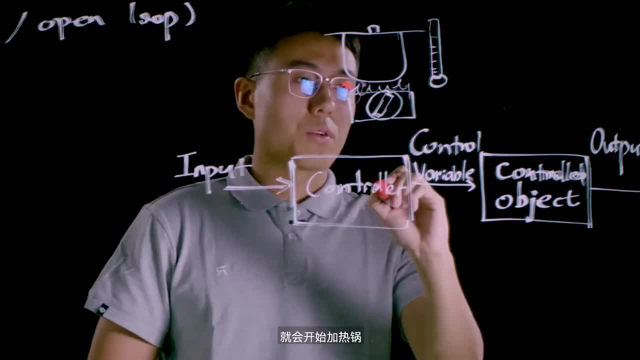 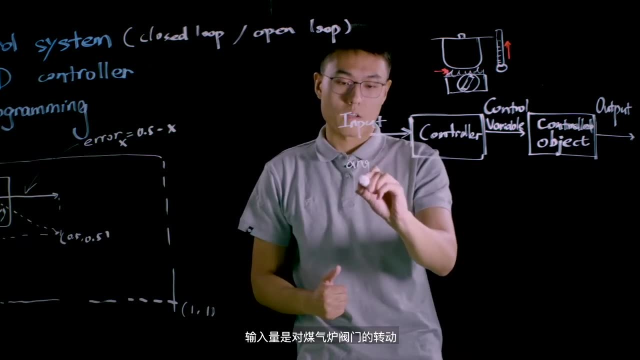 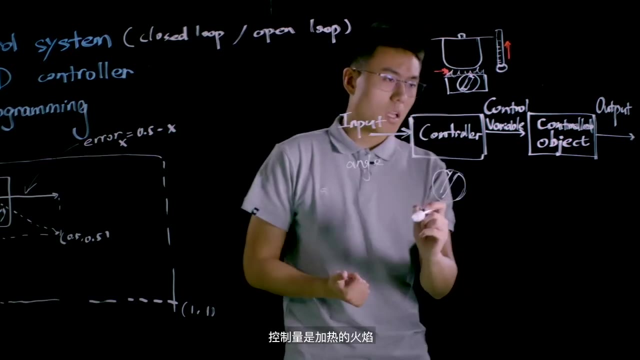 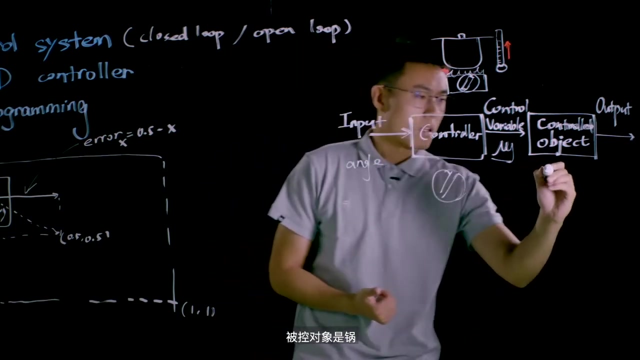 of the gas stove to produce flame, we start to heat the pot. So in this example the input is the angle of rotation And obviously the controller is the valve itself, The control variable is the flame And the control object is the pot. 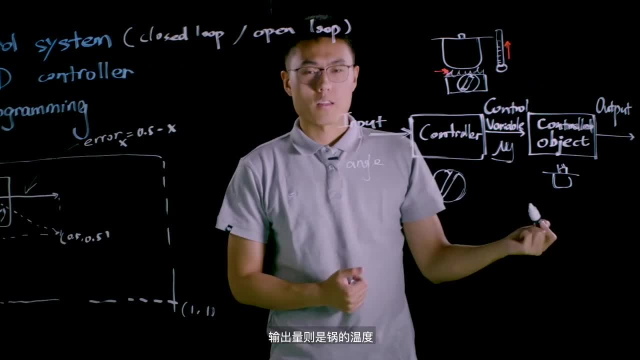 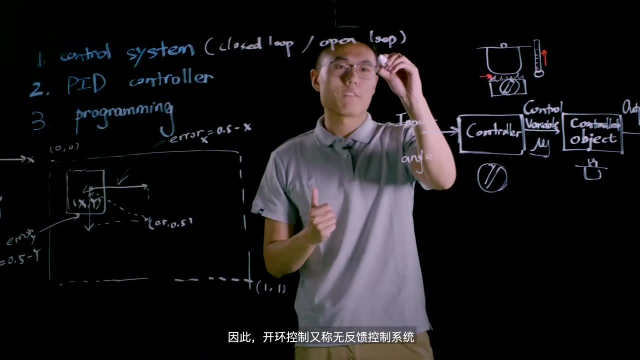 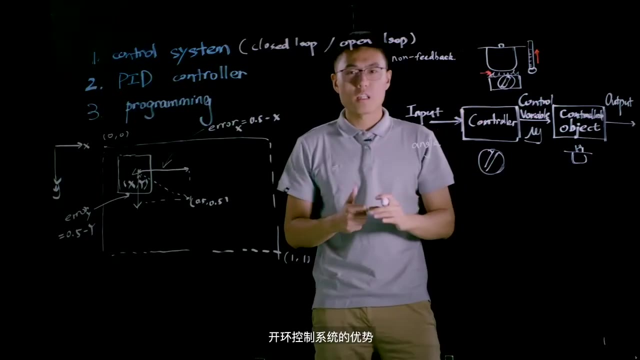 And the final output is the temperature of the pot. In this open loop system there is no feedback from the output value, So we also call this system a long feedback control system. The advantage of this open loop control system is it has simple structure. 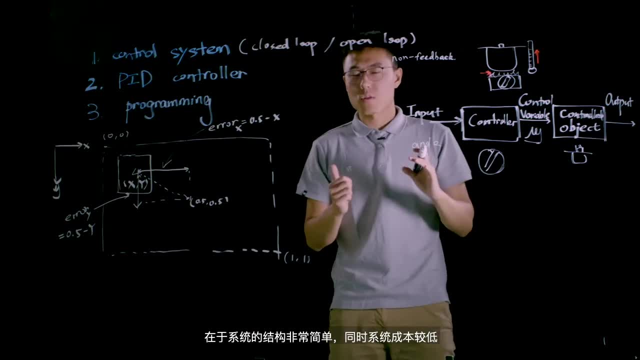 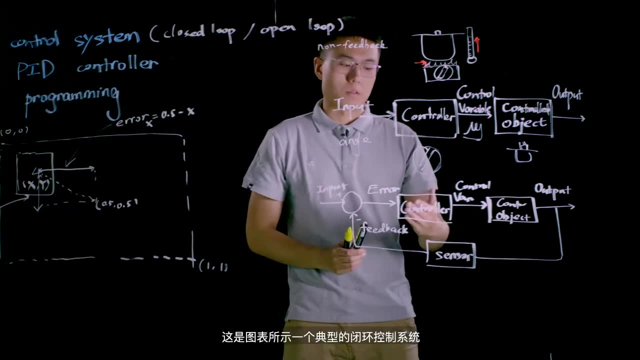 and very low cost. Let's take a look at the closed loop control system. Here is a diagram for the typical closed loop control system, Different from open loop control system. there is a sensor over here and it provides a signal path and forms a feedback loop. 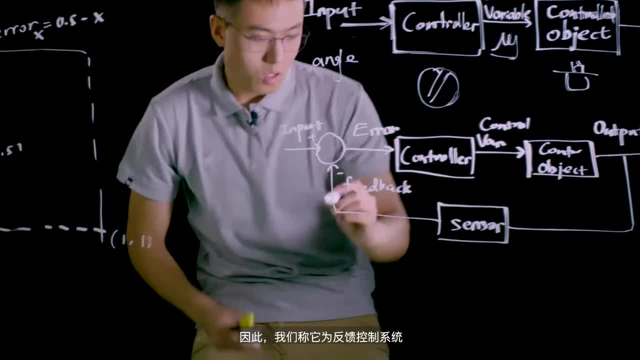 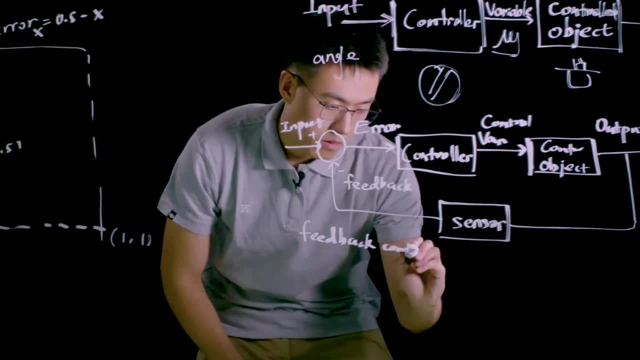 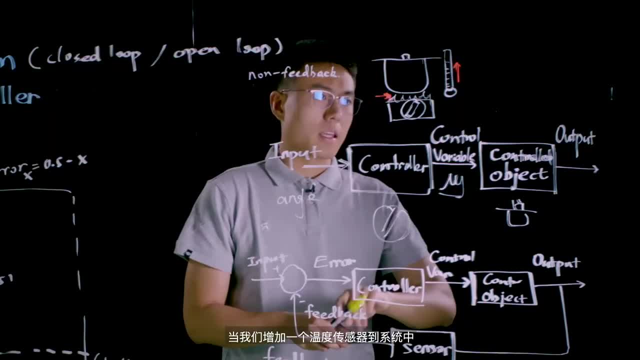 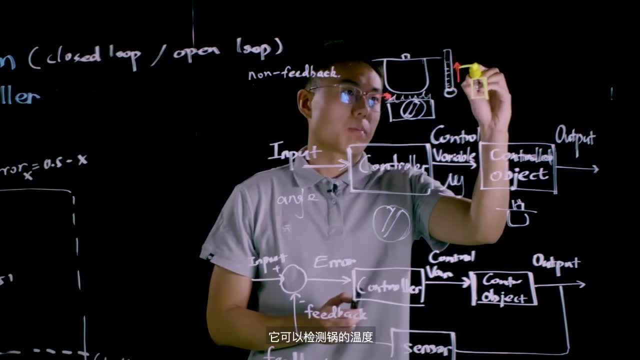 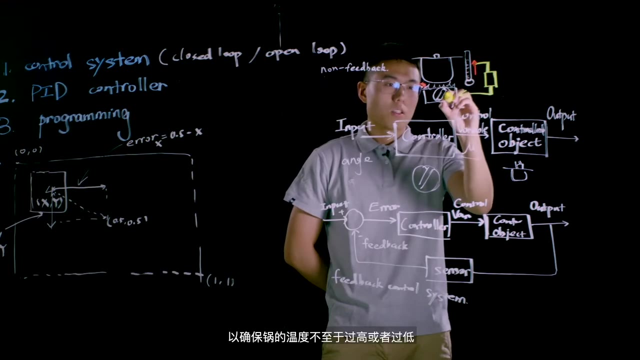 Now let's go back to the gas stove example. If we introduce a temperature sensor into this system and it can detect the temperature of the pot and provide it as a feedback to the system, it allows the stove itself to adjust the angle of the valve. 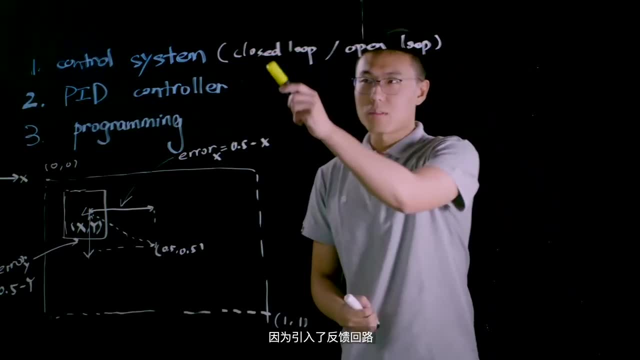 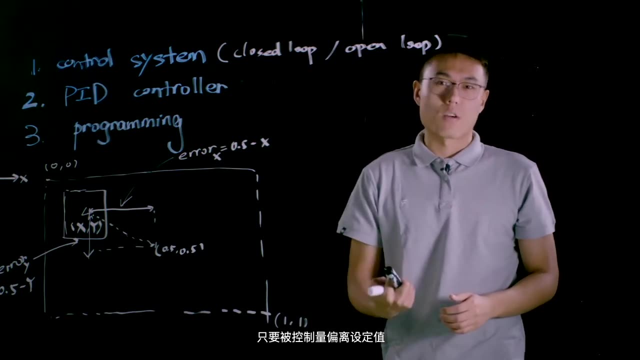 to ensure the temperature of the pot doesn't go too high or too low. This means the system has a feedback loop. It is structurally expensive and complex. As long as the output value deviates from the desired value, a corresponding control variable will be generated to eliminate the error. 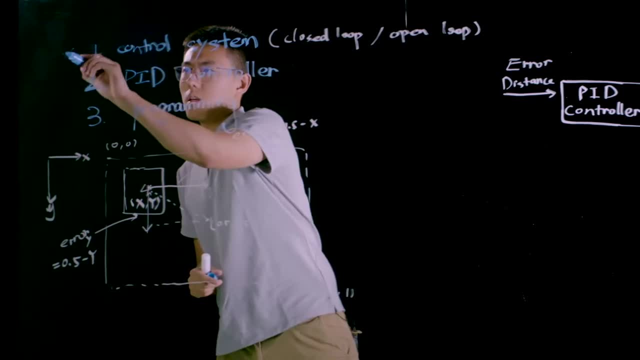 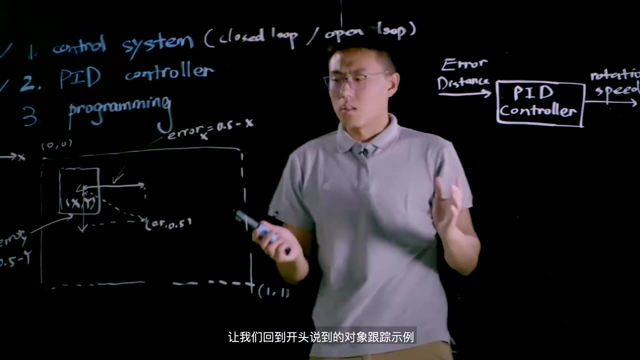 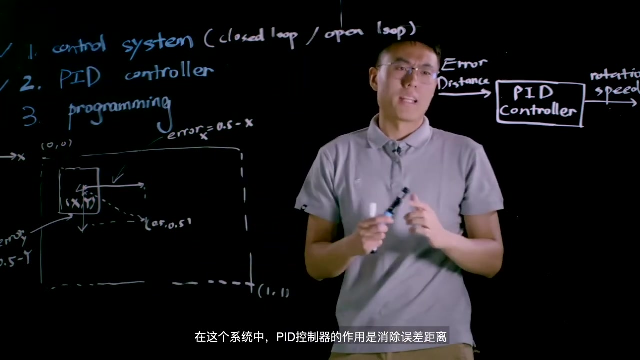 Now we understand what the control system is, Next we should learn something about the PID controller normally used in the control system. Let's go back to the object tracking example at the very beginning. The PID controller used in this system is responsible for eliminating the error at a certain distance. 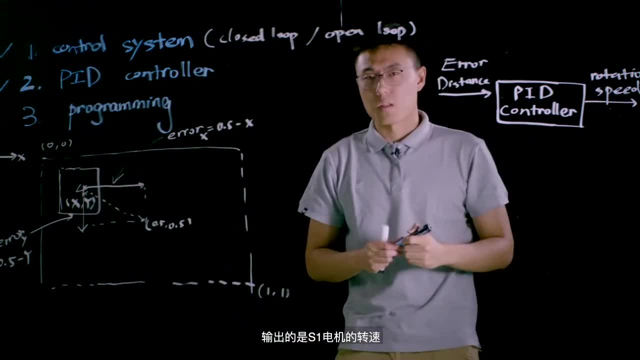 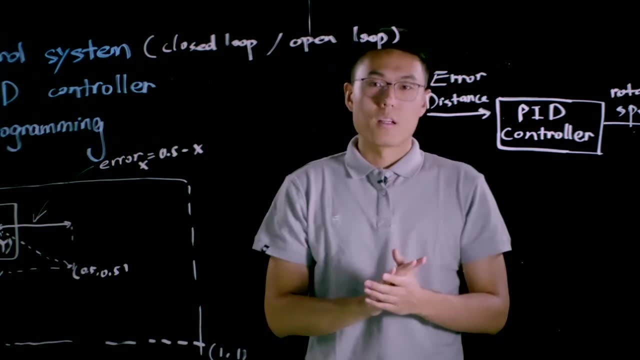 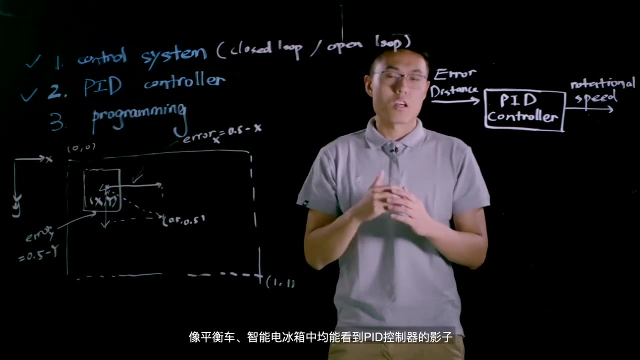 which is over here and output the rotational speed of the motors of S1.. There are two PID controllers governing the motion of Gimbal, one for pitch motor, another one for yaw motor. Actually, PID controllers are not only used in robot control systems. 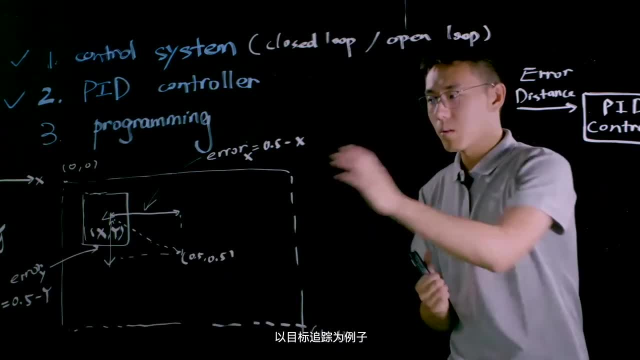 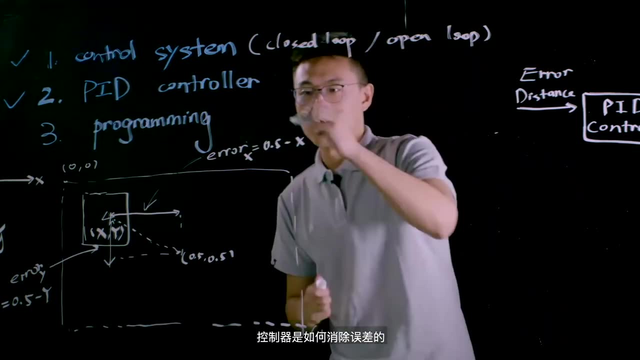 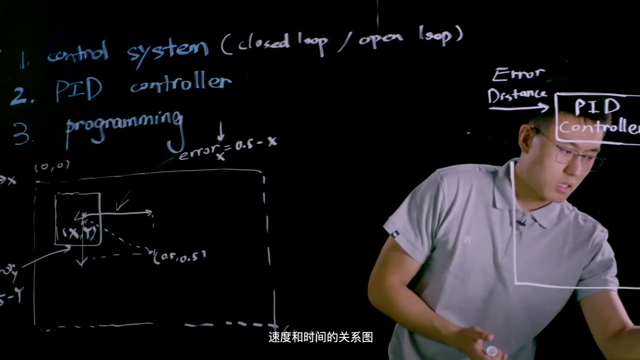 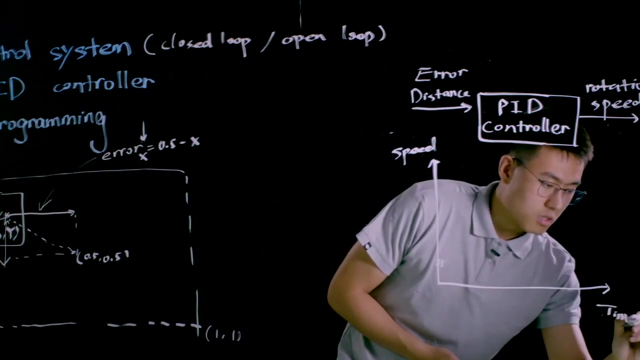 but also found in many other applications, such as smart refrigerators or hoverboards. So for the example of object tracking, we need to know how the PID controller works. First of all, we need to draw a graph of speed versus the time This speed is actually. 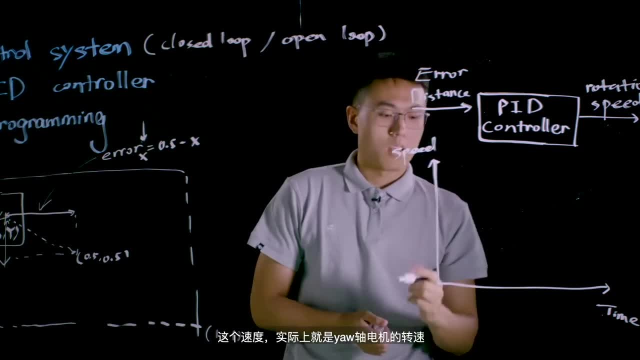 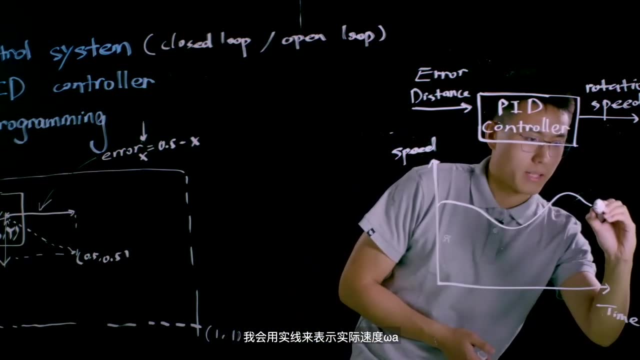 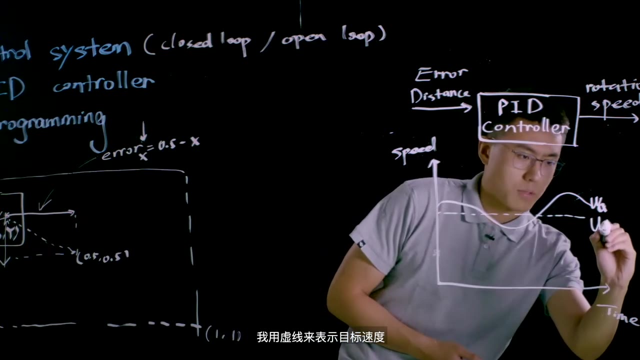 the rotational speed of the motor on yaw axis. I'll use a solid line to represent the actual speed- omega A- and I'll use a dashed line to represent the target speed or desired speed. omega D- PID controller can calculate three different outputs. 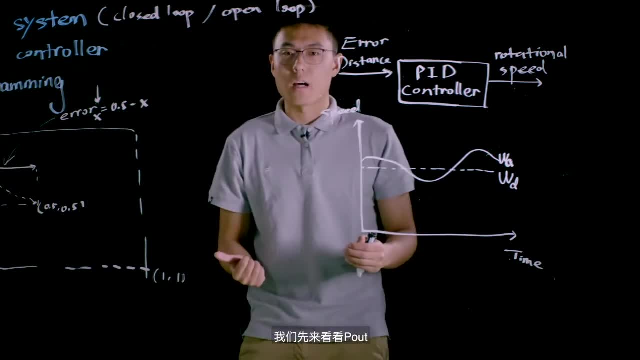 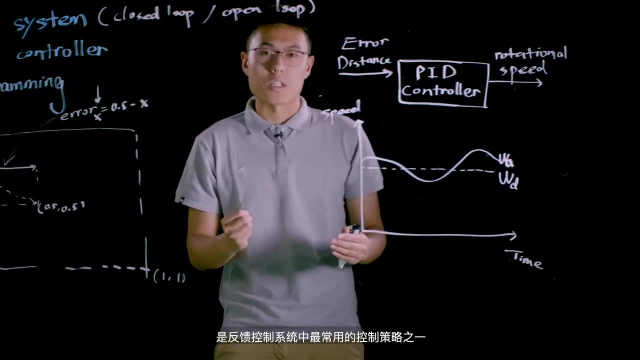 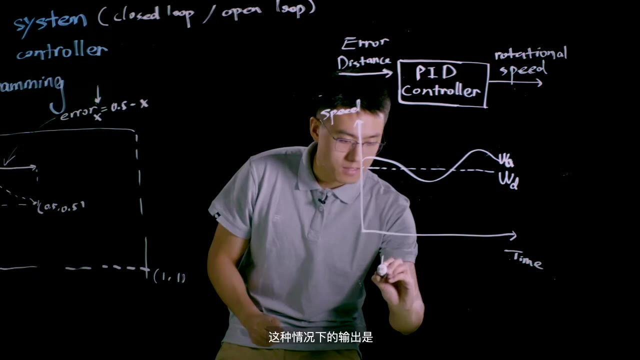 Pout, Iout and Dout. Let's take a look at the Pout first. P control, or proportional control, is one of the most frequently used control strategies in feedback control systems. P denotes proportional and the output under this case is. 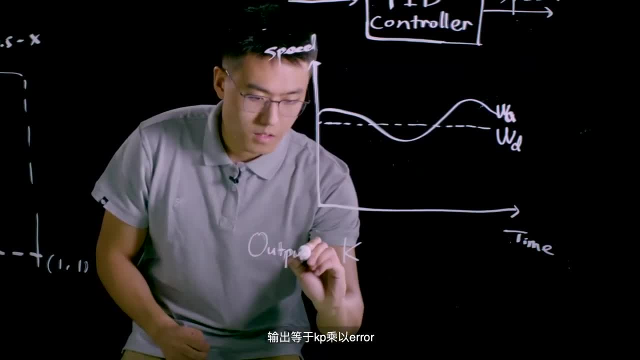 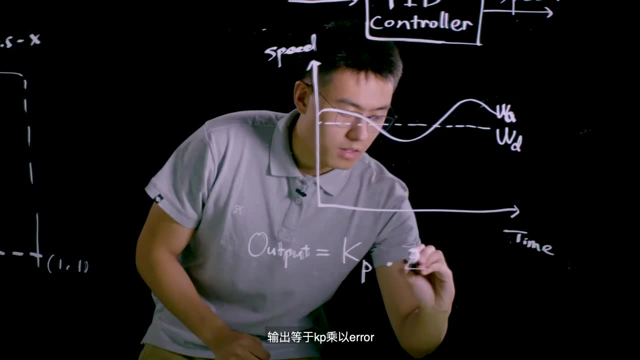 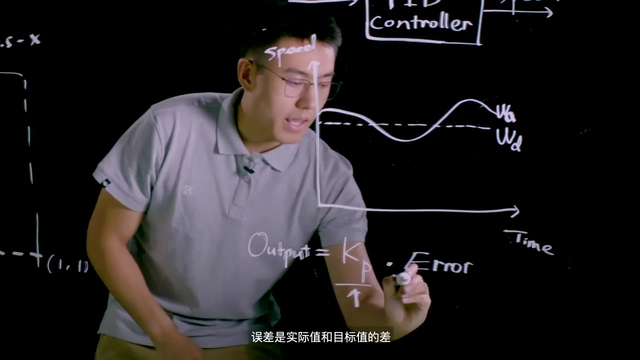 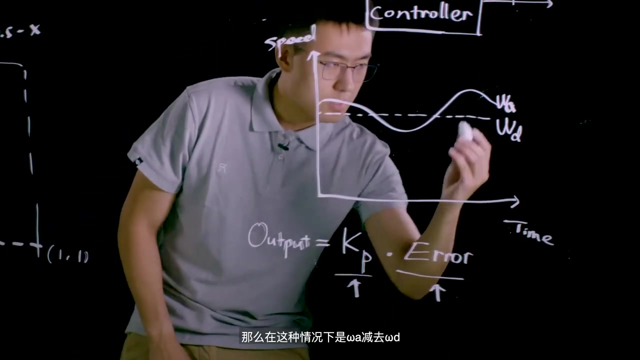 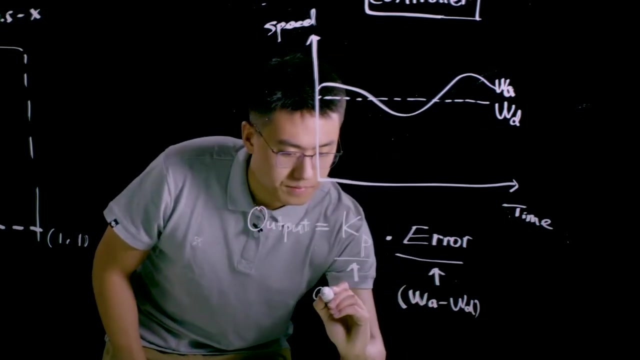 output equals to Kp times error Here. Kp is the scale coefficient And error is the difference between the actual value and the target value. So in this case it's omega A minus omega D. P is proportional to the error. 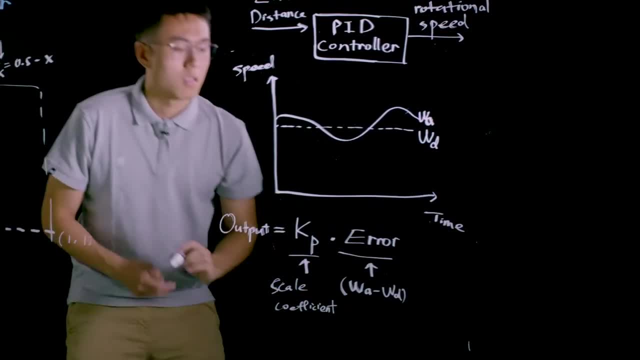 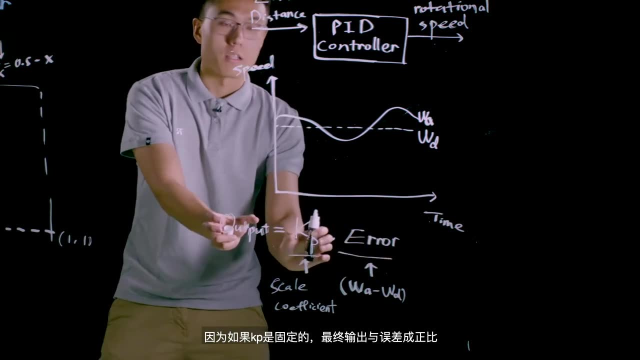 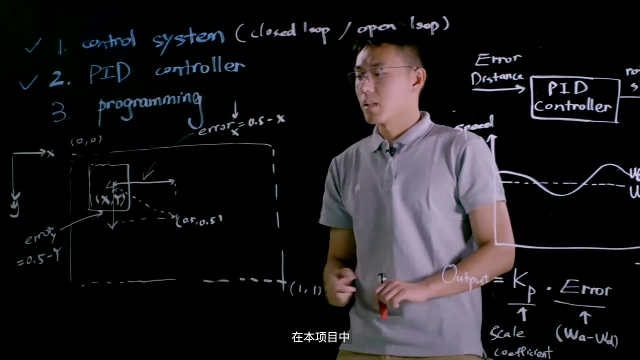 So we call it proportional control, because the final output is proportional to the error. if the Kp is fixed, And the greater the error is, the greater the output will be In this project. when the center of the viewport is approaching to the desired position. 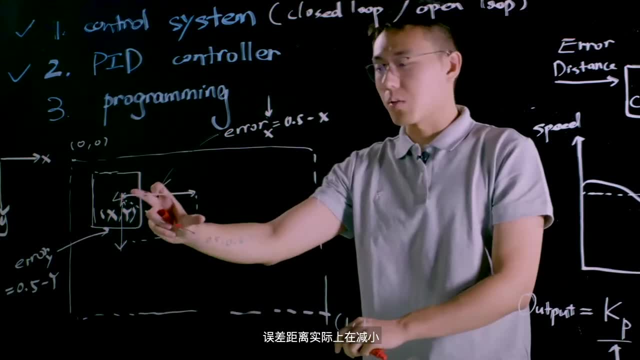 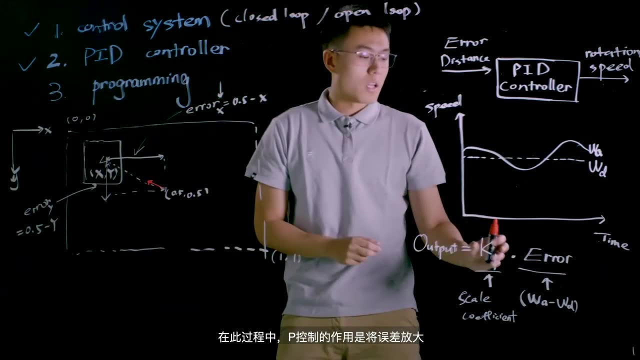 which is the center of the visual marker. error distance is actually decreasing And at the same time, the rotational speed of the motor is dropping as well. During this process, the function of P control is to amplify the error and convert it into the output. 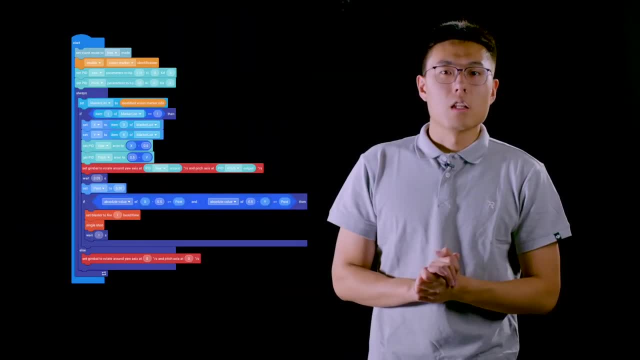 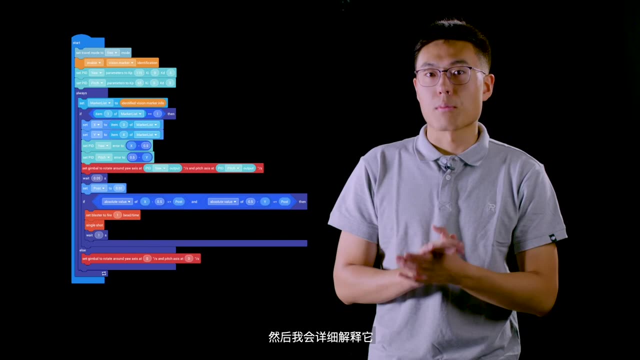 of rotational speed. Great, it's time to do some programming. The following program allows Gimbal to track the visual marker. Let's first take a look at how the program works and then I will explain the program in detail. If we increase. 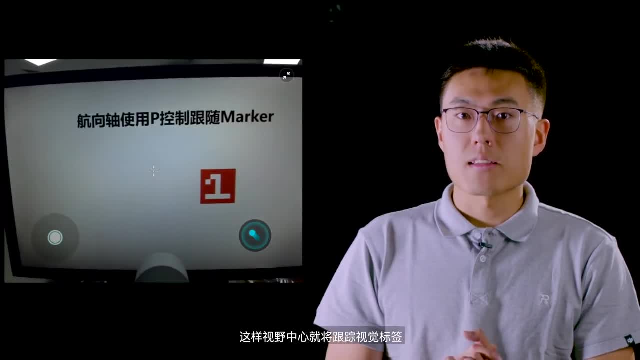 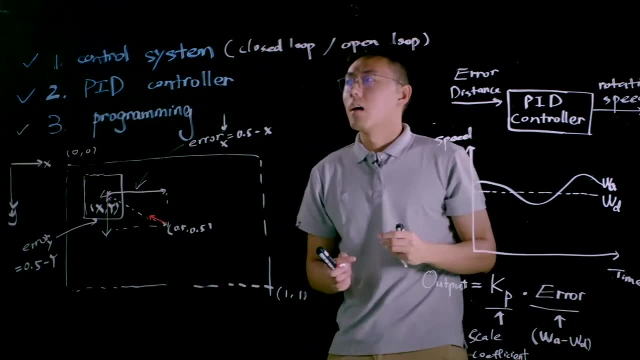 the Kp parameter, the Gimbal will accelerate faster so that the center of the field of view of the camera will track the visual marker. Now let's do a very quick recap of today's lesson. First of all, we learn what the control system is.